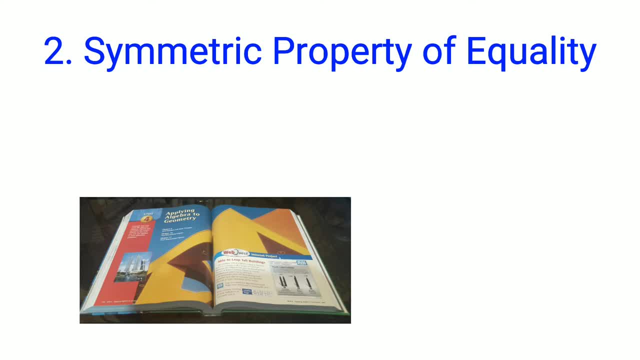 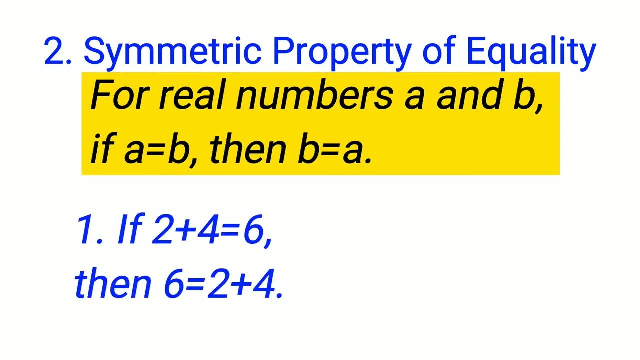 property is called symmetric property of equality. Look at this book. Both sides are equal or symmetrical For any real numbers, A and B. if A is equal to B, then B is equal to A. For example, number 1,: if 2 plus 4 is equal to 6,, then 6 is equal to 2 plus 4.. Example: 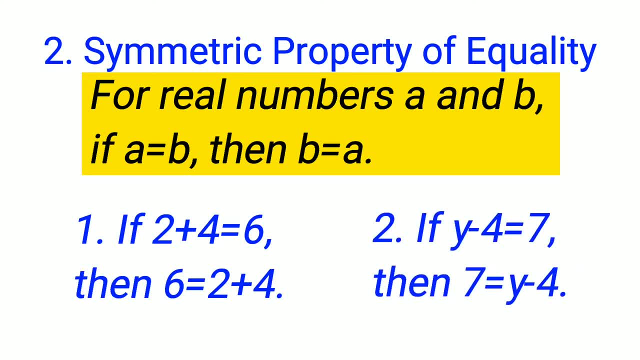 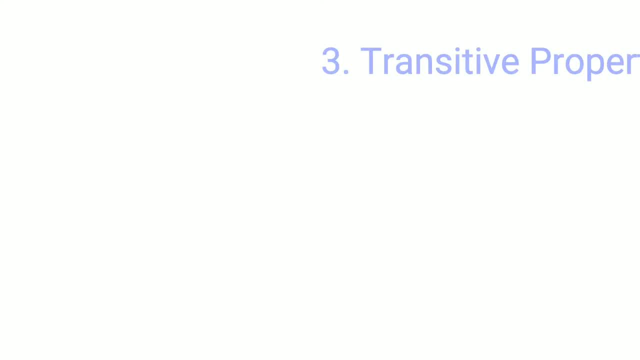 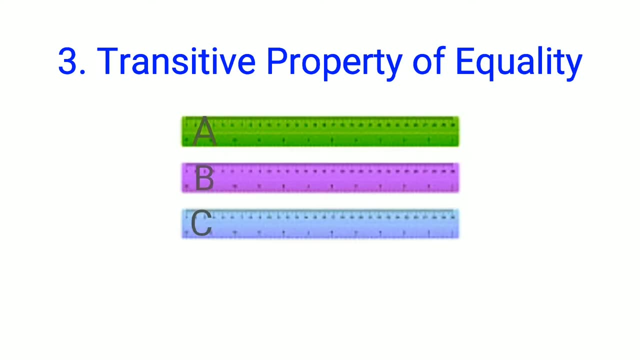 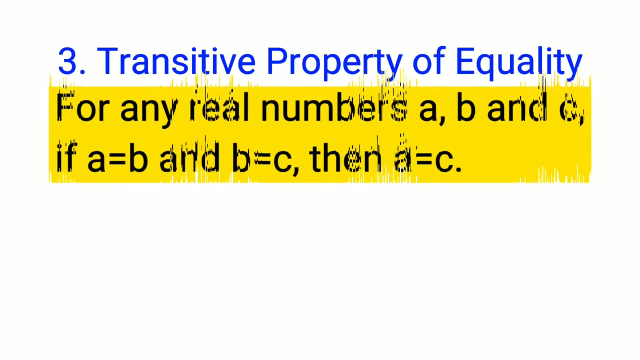 2,. if Y minus 4 is equal to 7, then 7 is equal to Y minus 4.. The third property is called transitive property of equality. This property is like these three rulers of different colors, yet all of them are equal For any real numbers: A, B and C. 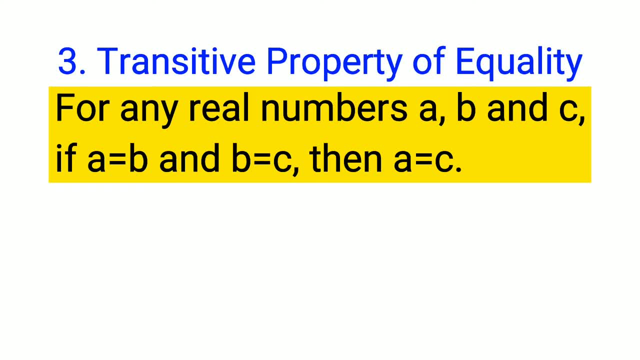 if A is equal to B and B is equal to C, then A is equal to C. For example, number 1, number 2, number 3 is equal to 3 plus 4 is equal to 7 and 7 is equal to 5 plus 2.. If 3 plus, 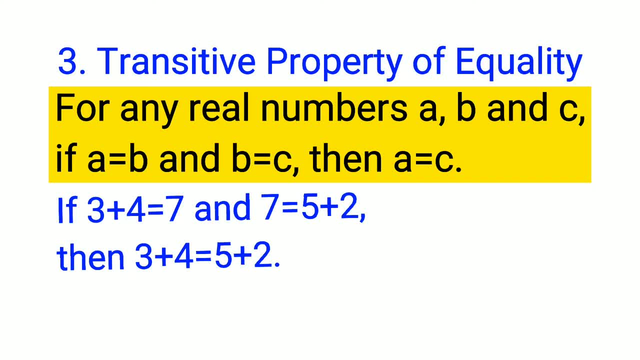 4 is equal to 7 and 7 is equal to 5 plus 2, then 3 plus 4 is equal to 5 plus 2.. Another: if X plus 5 is equal to Y and Y is equal to 8, then X plus 5 is equal to 8.. The fourth: 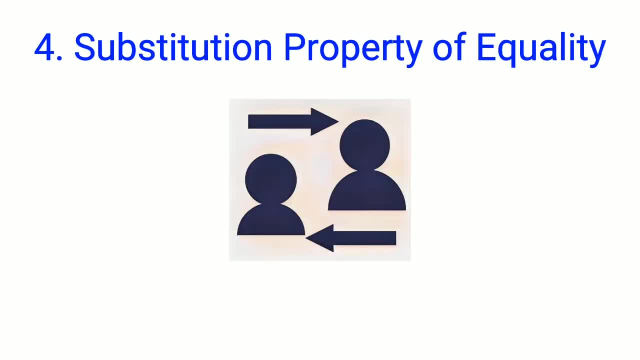 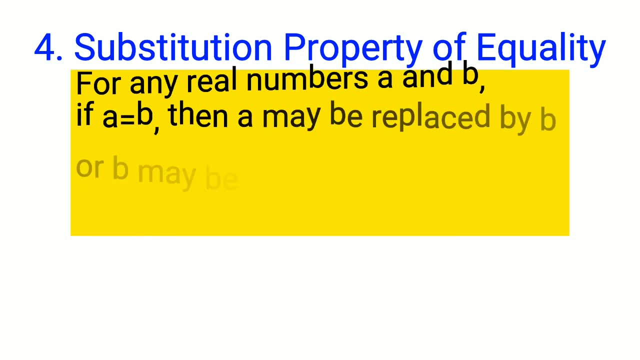 is substitution, property of equality. This is like substitution in basketball or any game of chess. If the game of chess is equal to 3 plus 4, then 3 plus 4 is equal to 7.. If game where one can be replaced by another For any real numbers, A and B, if 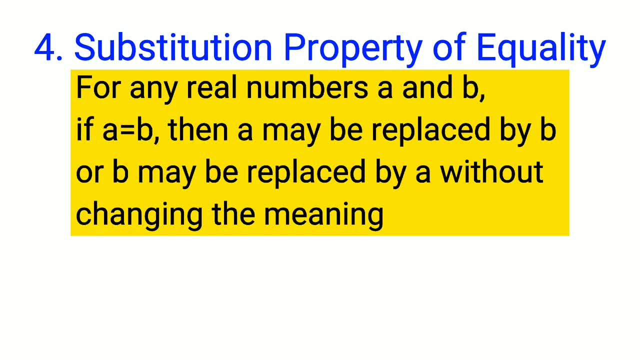 A is equal to B, then A may be replaced by B or B may be replaced by A without changing the meaning. For example, if X plus Y is equal to 10 and X is equal to 4, then by substitution 4 plus Y is equal to 10.. The fifth is called addition. 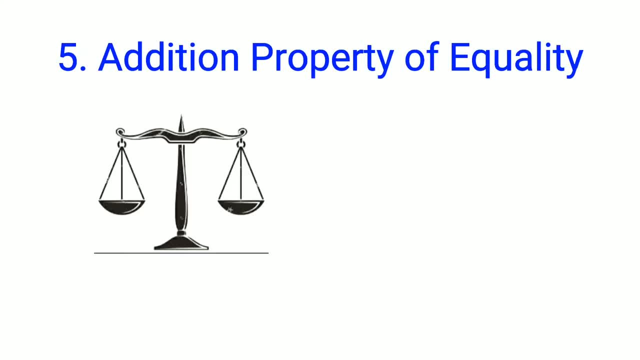 property of equality. This weighing scale is balanced because both sides have equal weights. If we add more weights in only one side, it's no longer balanced. To make it balanced, add both sides equal weights. If A is equal to A and C is equal to D, then A plus C is equal to D. 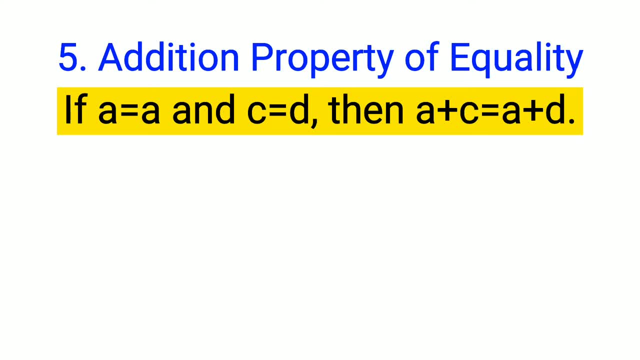 Example 1: if 6 is equal to 6 and 10 is equal to 3 plus 7, then 10 plus 6 is equal to 3 plus 7 plus 6.. Simplifying 16 is equal to 16.. Solve X minus 4 equals 0.. 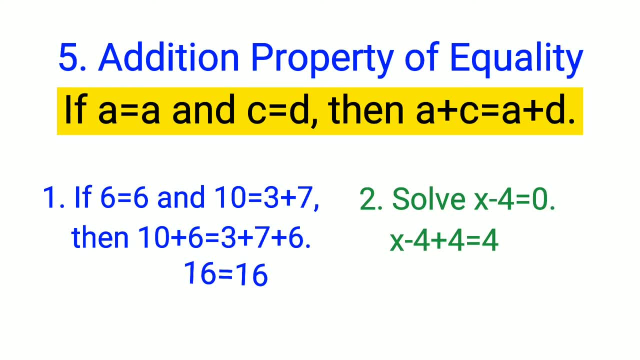 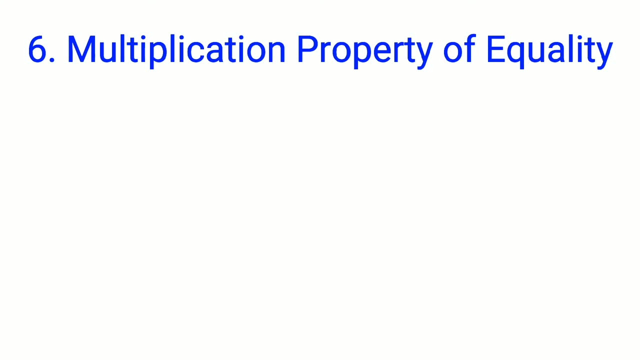 Add both sides by 4, we have X minus 4 plus 4 is equal to 4.. Simplifying: we have x is equal to 4.. The sixth one is called multiplication property of equality For all real numbers, a, b and c. where c is not equal to 0, a is equal to b if and. 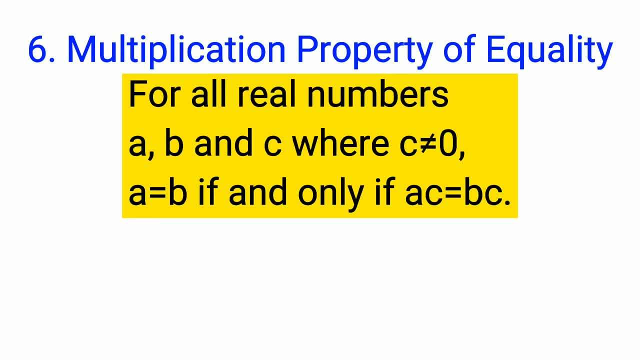 only if ac is equal to bc. Let's put this simply by these examples. Number one: 4 times 3 is equal to 12.. This can be multiplied both sides by any number, say 5.. We can have: 4 times 3 times 5 is equal to 12 times 5.. 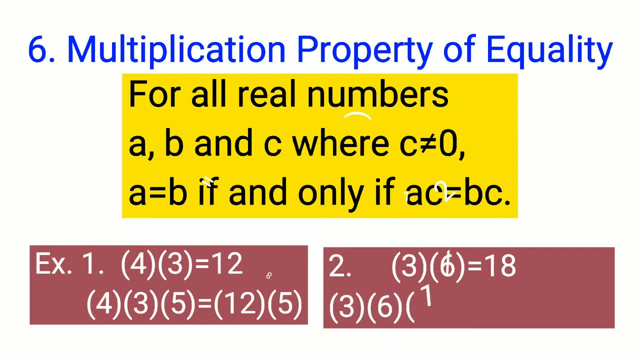 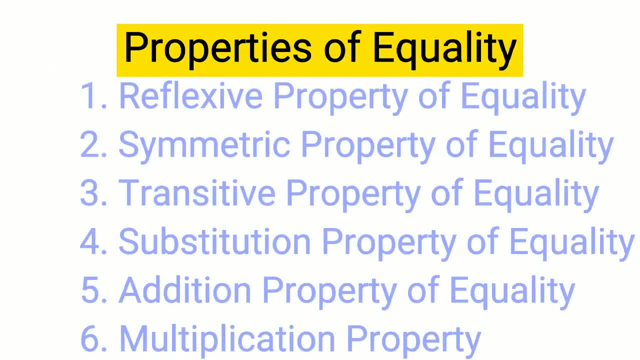 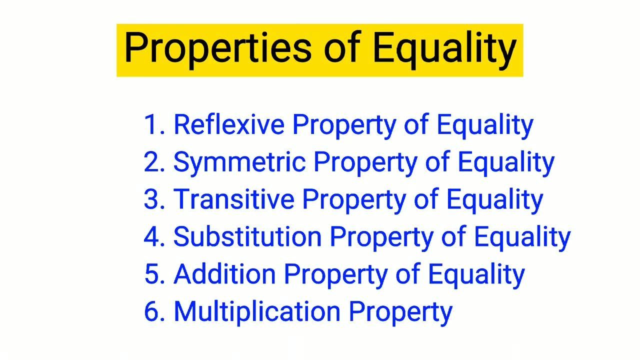 Example number two: 3 times 6 is equal to 18.. We can multiply both sides of the equation by one, half or any number. We only have six properties of equality. Notice here that we don't have any properties of equality. We do not have subtraction property and division property. 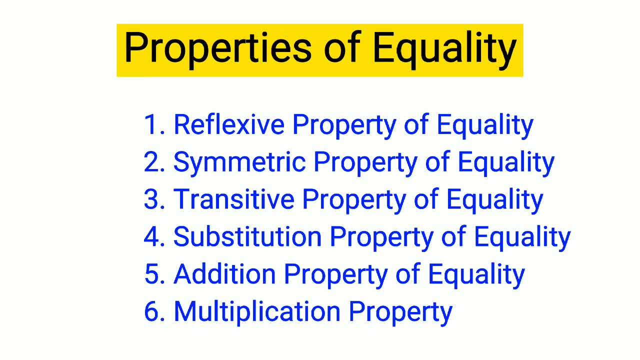 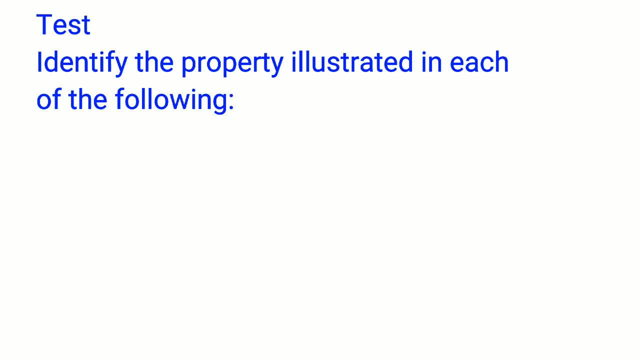 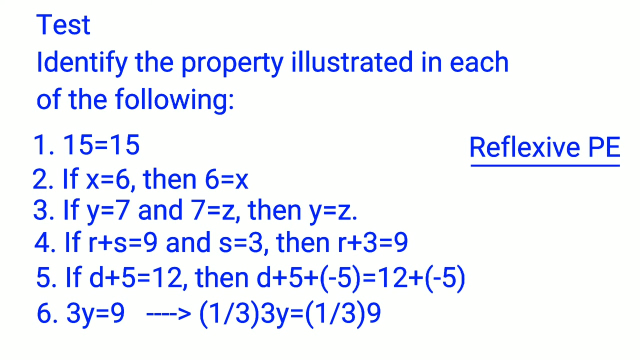 Subtraction is already incorporated. in addition, while division is incorporated in multiplication property of equality, When you multiply both sides and have divided the two corners, the theoremç becomes minus one half. That's why N is here. loral integral should be less than n, but the halving of n is smaller than n. 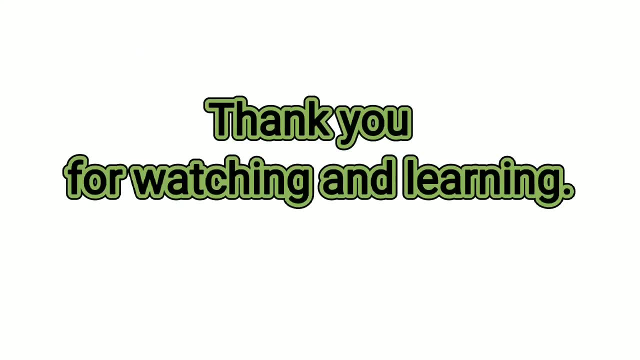 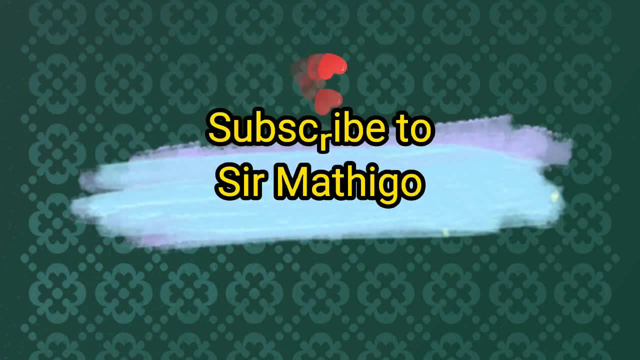 and valued neutral của. We have x out of 5.. Thank you for watching. See you tomorrow.